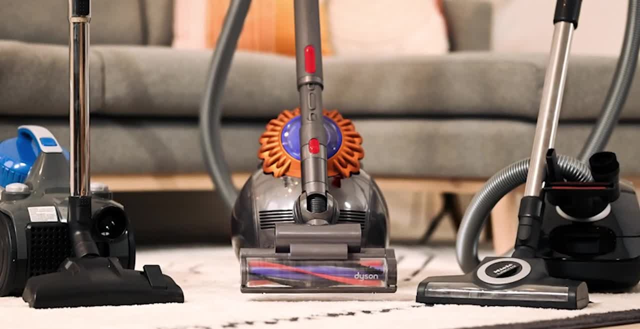 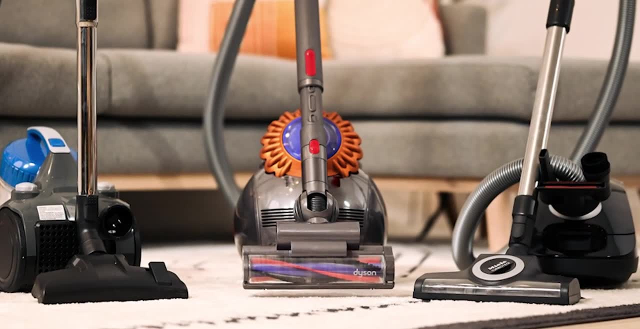 Therefore, in terms of function maximization, the canister vacuum has an edge, since it offers more cleaning functions. Storage: A canister vacuum takes more space as it comes in separate units, And the hose is not stable enough to stay upright and keeps falling over. 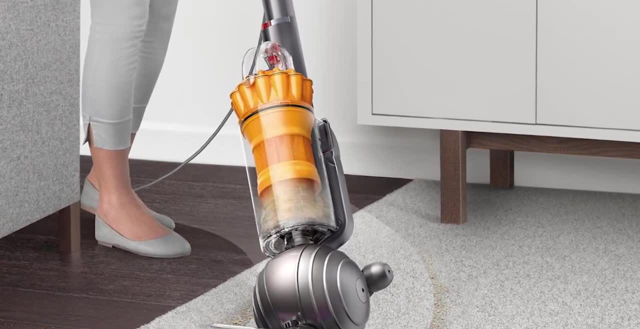 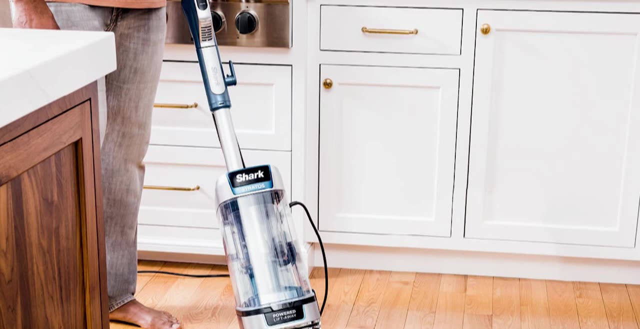 The upright vacuum comes in a single unit and stays upright, And some even have a storage mount that you can fix on the wall, allowing you to save on space. So, in terms of storage management, the upright vacuum takes the lead because it's easier to store. 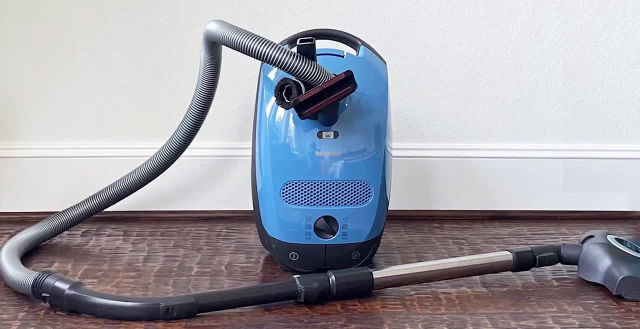 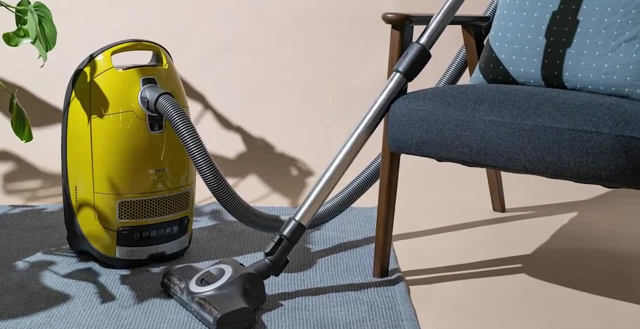 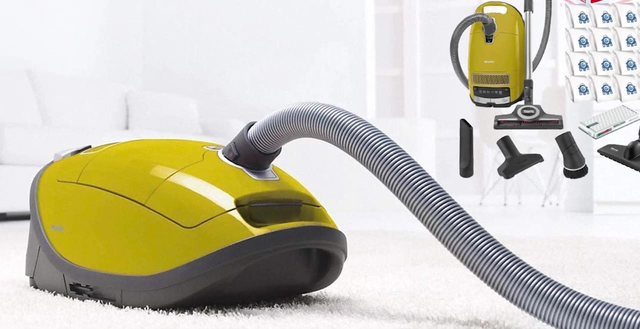 Comparison Table. From the table. a canister vacuum is quieter, which could make it a good choice for a household with kids. as opposed to the upright vacuum Comparison Table, The canister vacuum also weighs less, making it lighter to use. However, despite the upright vacuum being heavier, it doesn't require lifting off the 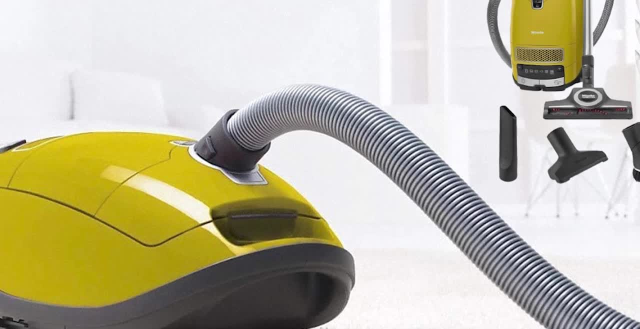 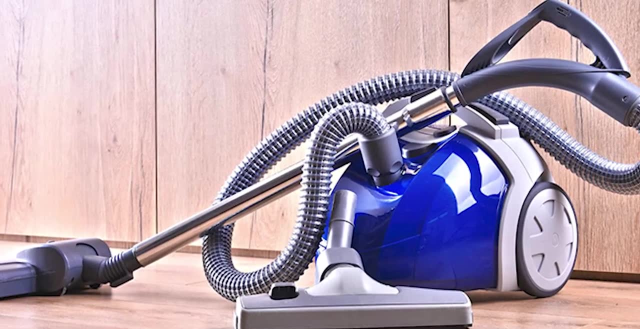 ground during operation and you might only feel the weight after using it for a while. Similarities: Both canister and upright vacuums are great carpet cleaners. The suction power of the canister allows it to suction all the debris in the carpet. 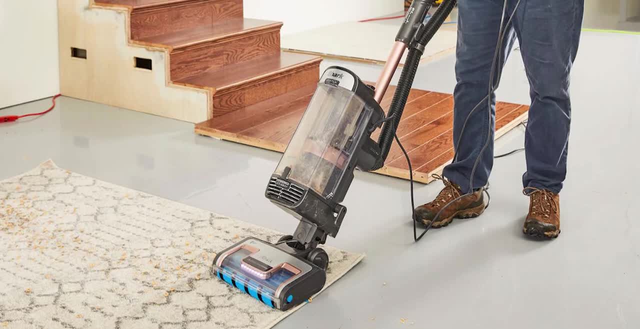 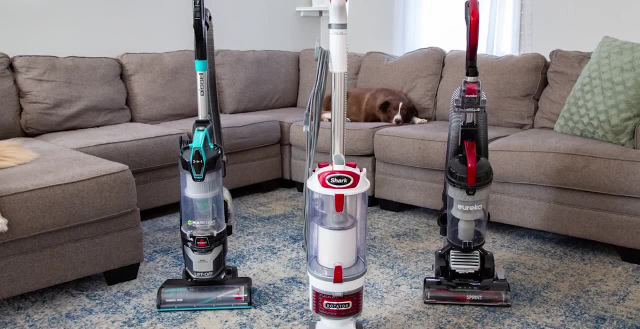 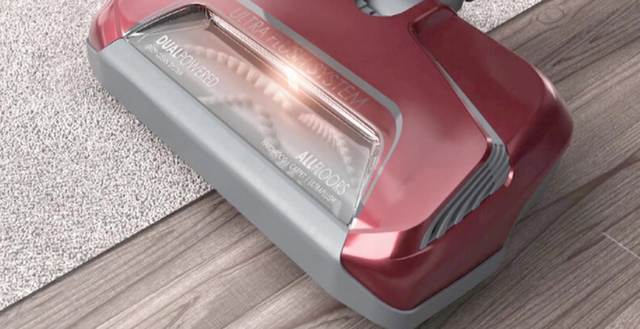 while the motorized brush on the upright vacuum allows for carpet deep cleaning by agitating the carpet fibers, thus lifting off the dust and dirt. Verdict Which is the right one for you. Both canister and upright vacuum cleaners have their perks. Therefore, selecting the right fit for you would depend on your specific needs. 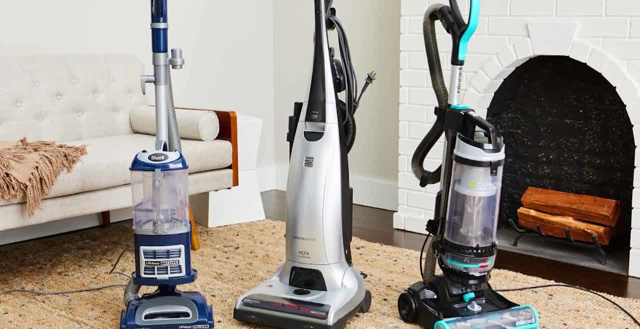 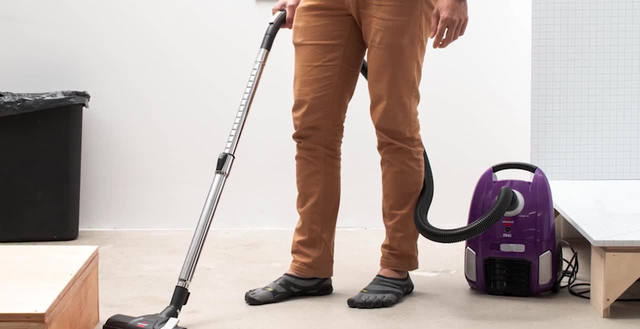 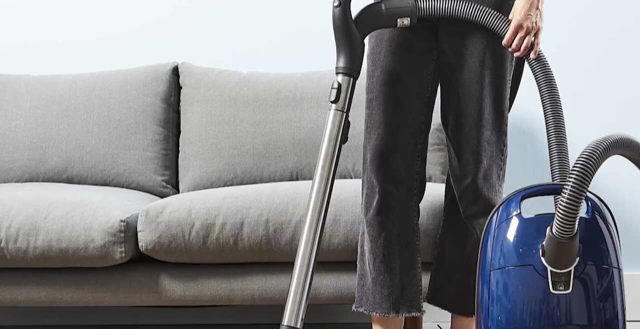 The upright vacuum is an excellent option for large areas and carpets due to its wide floorboards and mechanical brush. For tight spots such as stairs, corners and your upholstery and a household with kids, the canister vacuum is the best option. If you liked this video, please hit the thumbs up button and subscribe to our channel. 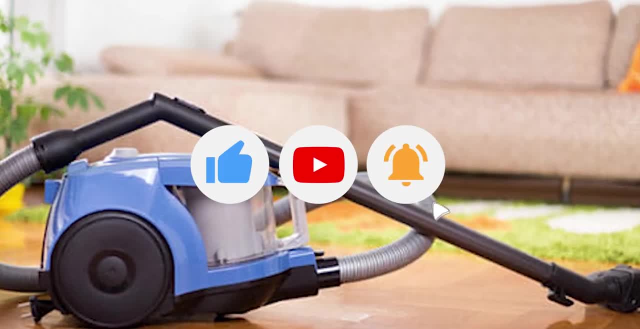 Also, let us know which other comparisons that you would like to see next from us.